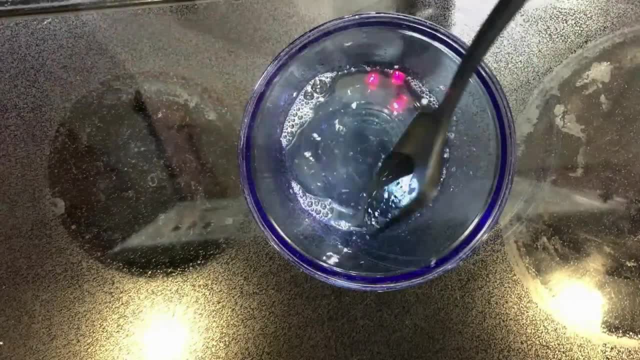 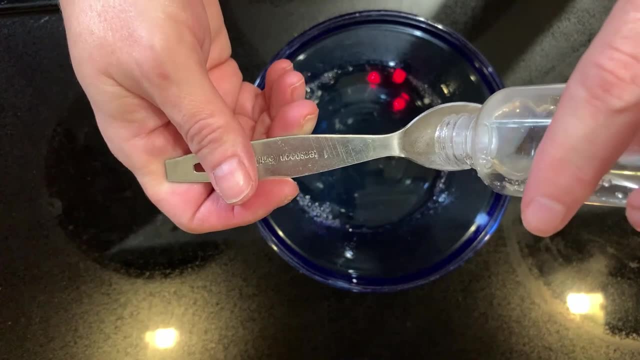 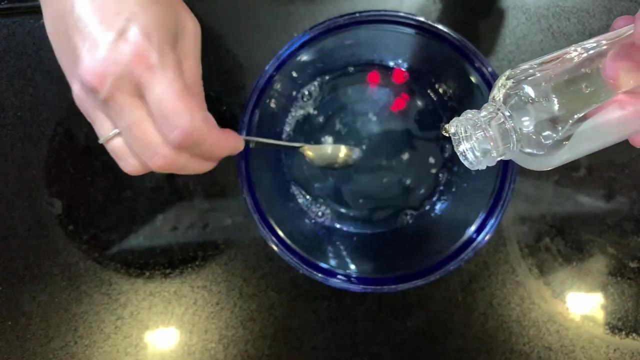 Once the gelatin is completely dissolved in the water, add two teaspoons of corn syrup. Heating your container of corn syrup in your mug of hot water helps make it easier to pour. However, it is still very thick and you'll have to have patience. 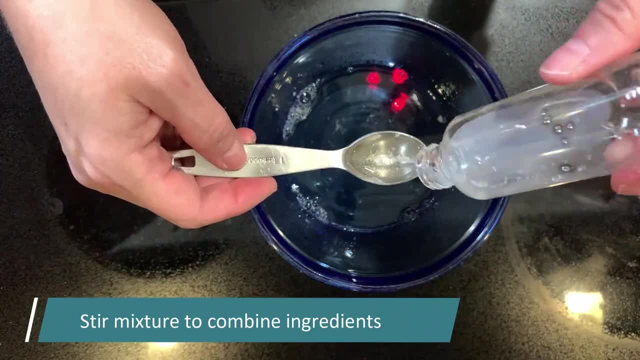 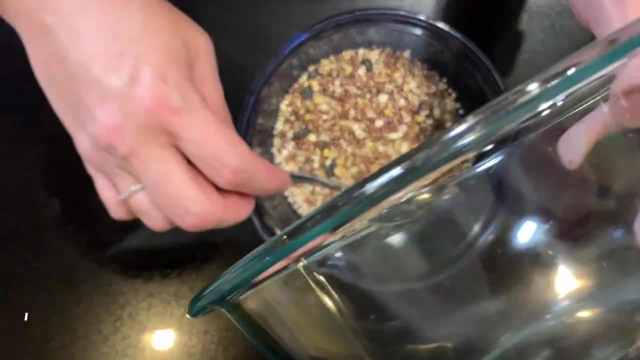 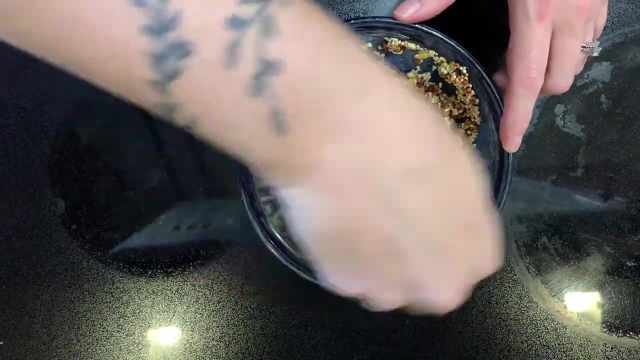 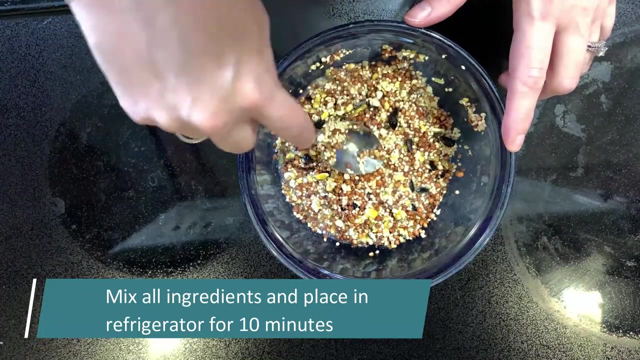 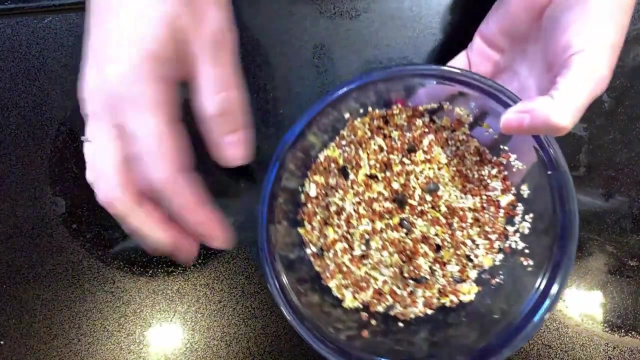 Stir the mixture well to combine all of the ingredients. Next add your cup of bird seed. Mix well and put in the refrigerator to set for 10 minutes. After 10 minutes, take your bird seed out of the refrigerator. It should be firm to the touch. 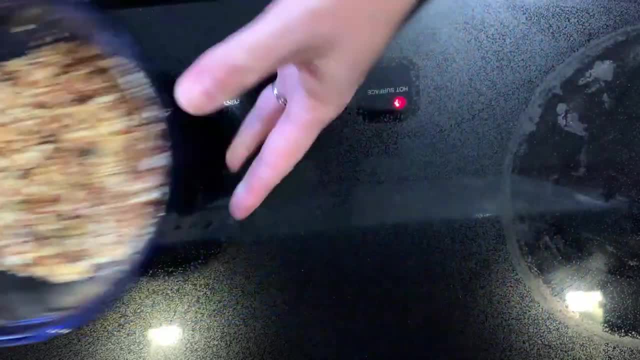 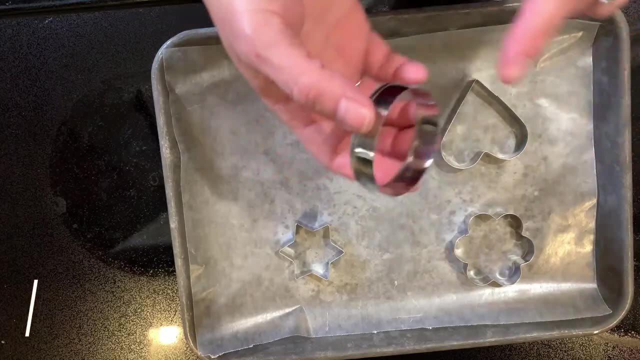 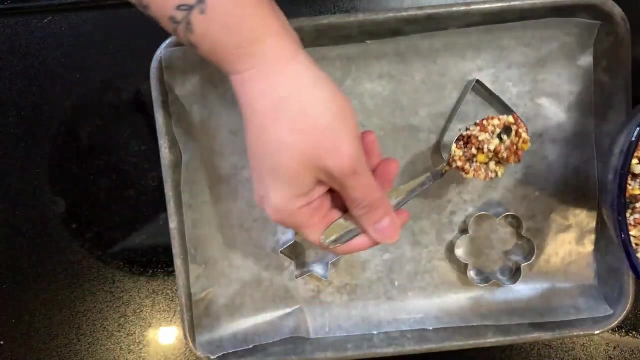 Now we're ready to begin filling our cookie cutters with bird seed. It's important to make sure and place the sharp edge of your cookie cutter down on the parchment paper Using a spoon. fill your cookie cutters with the bird seed mixture. 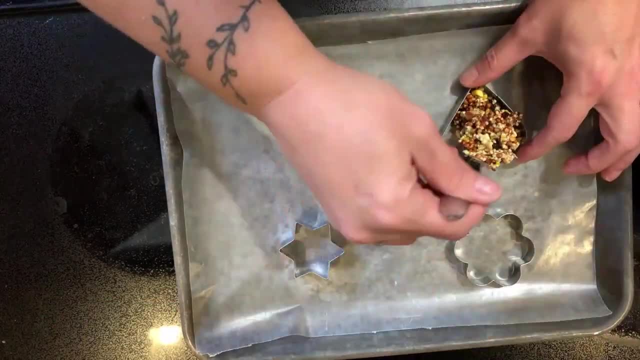 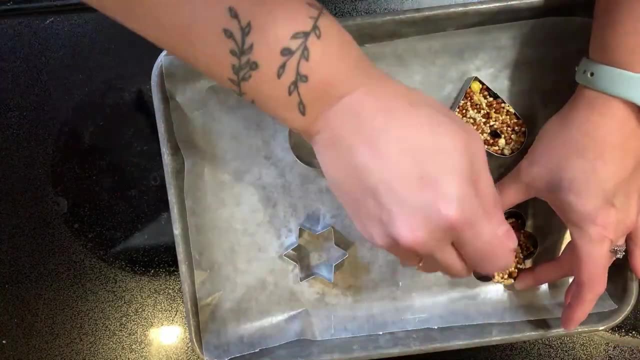 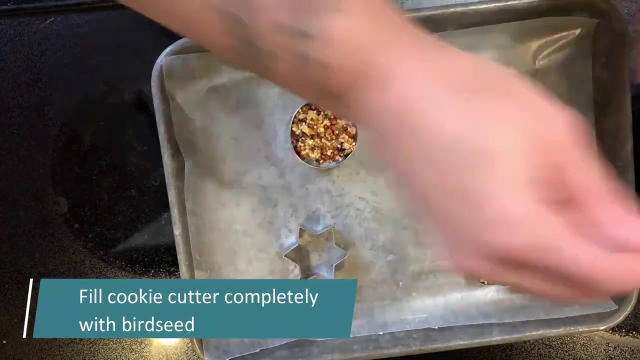 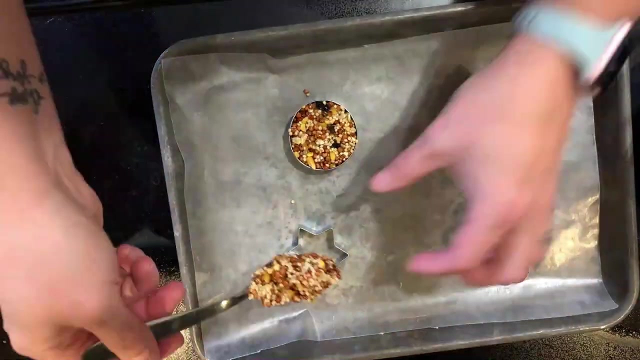 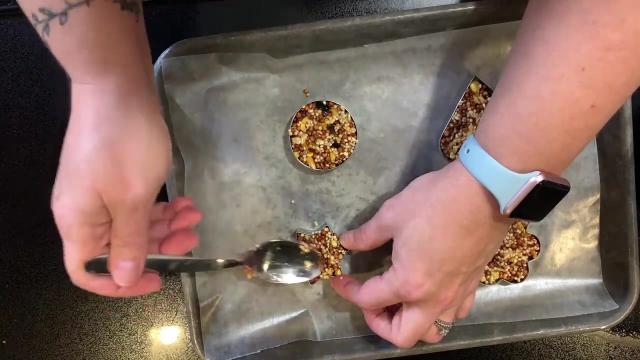 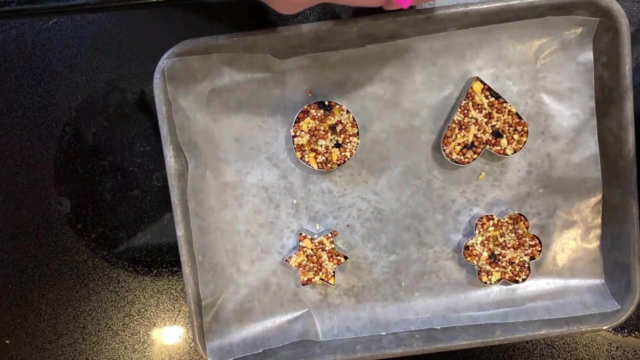 Make sure to tap the cookie cutter to make sure it's not sticking to the bottom of the container. Make sure to tap the cookie cutter to make sure it's not sticking to the bottom of the container. Make sure to tap the bird seed mixture into all the little corners and crevices of your cookie cutter. 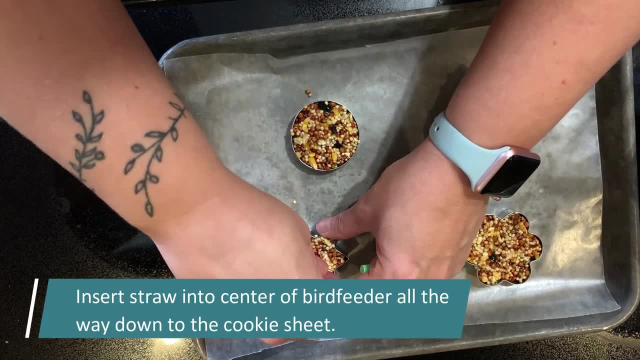 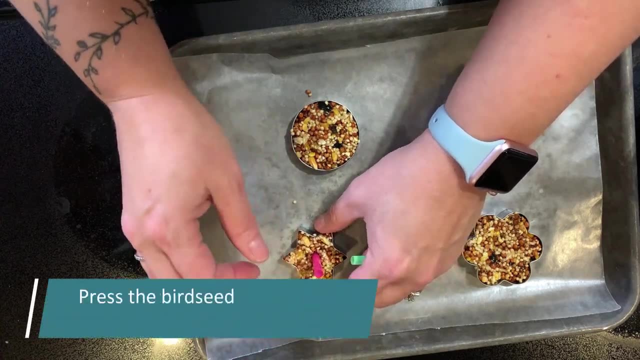 Take your straw and place it into the center of each bird feeder, working it all the way down till it touches the parchment paper on the cookie sheet. Pack the bird seed around the straw and into the corners of the cookie cutter so that it is firm. 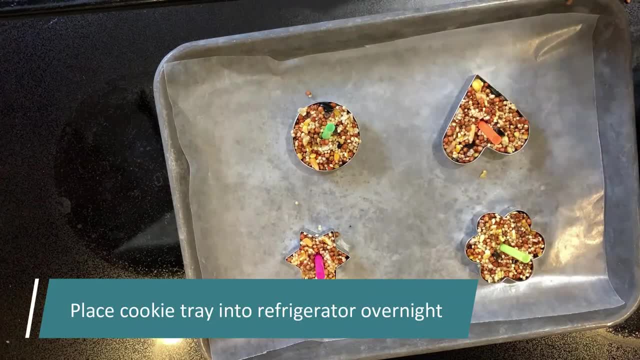 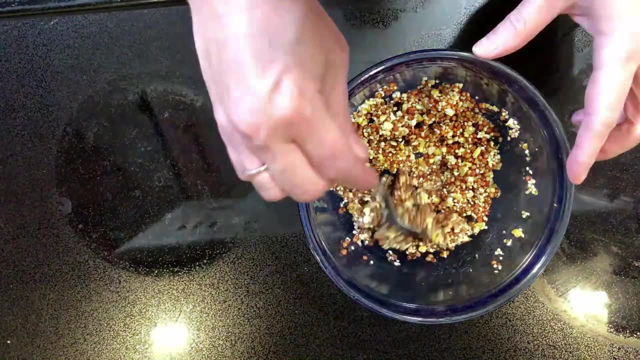 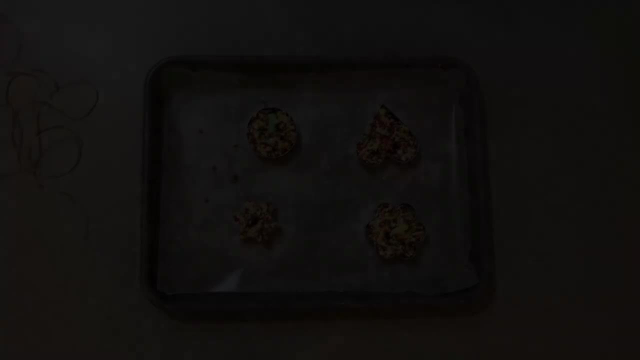 Once you have done this for all four of your bird feeders, you will place them in the refrigerator overnight to harden. With your extra bird food you can fill extra cookie cutters or even use paper cups as molds After letting them set overnight.